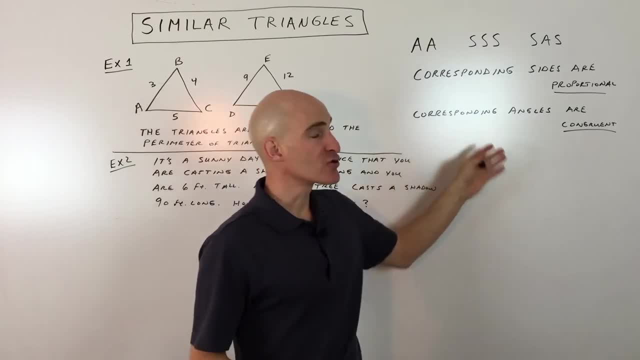 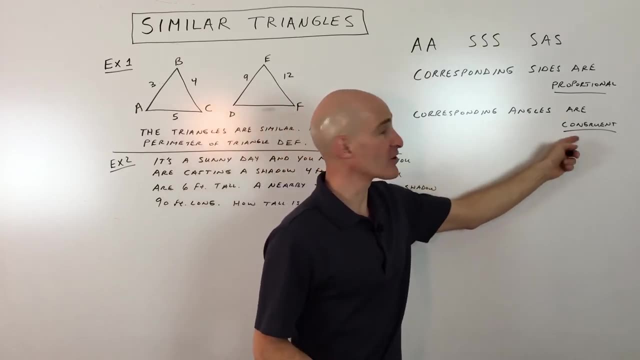 does that mean? Well, first of all, what it means is that the triangles, they have the same shape, but not necessarily the same size. So what that means is that the corresponding angles are congruent, but the corresponding sides, meaning the sides that match up, they're proportional. So 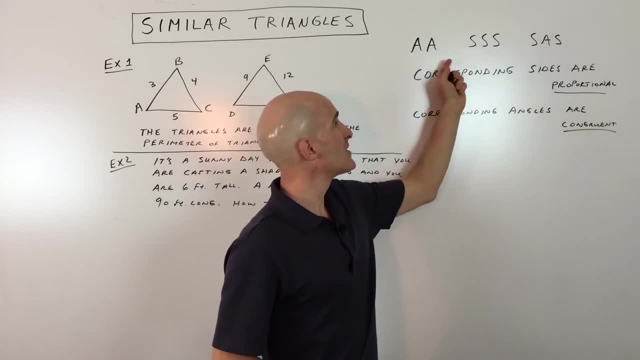 you might have remembered from your geometry class that you can show that triangles are similar by either using the angle angle similarity or the side side side, or the side angle side, and we'll go through that in a just in a brief moment here. So, basically, what we want to do is we want 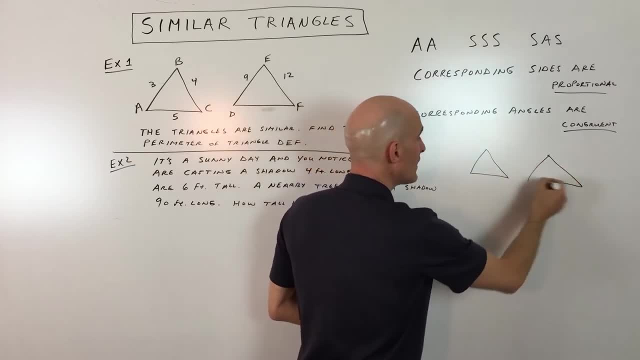 to look at the two triangles. So say, your triangles look like this and say, for example, that this angle and this angle are congruent, and angle and this angle are congruent. what you can see then is that automatically, the third angles will also be congruent and these triangles are then going to be. 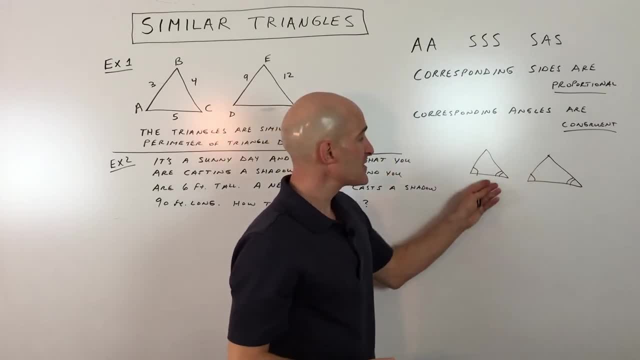 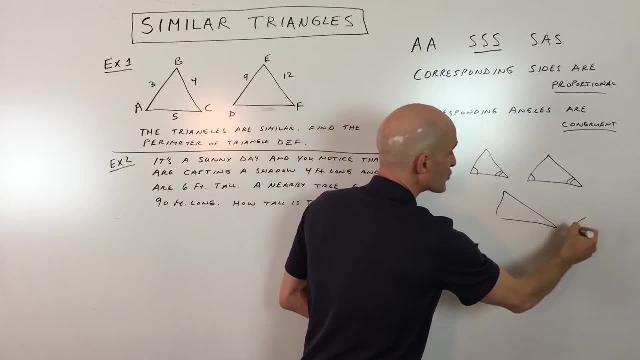 similar, meaning that the corresponding sides are proportional. So this is the form that it usually comes up in, but it also can come up in this side-side-side form, where you have three sides of one triangle are in the same ratio as three sides of another triangle, For example, like this might be: triple this side and 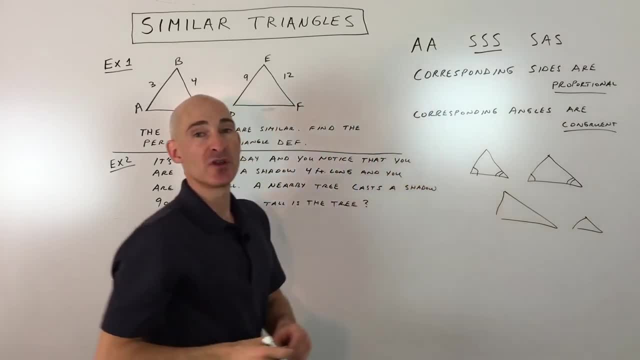 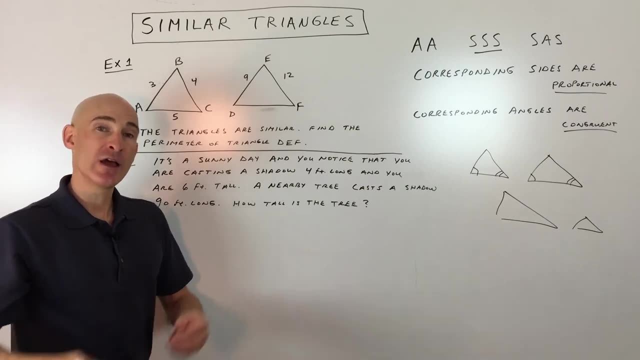 this might be triple this side, and so on. So let's go into the the first example here. Now, what I'd like for you to do is go ahead and pause the video, see if you can solve this problem yourself, and then go ahead and, you know, check your answer. 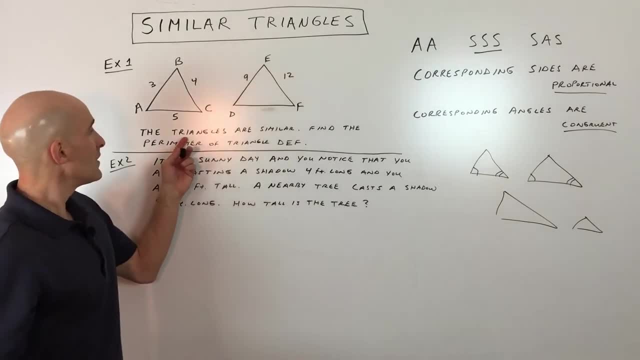 when we go through it together. So first of all, it says the triangles are similar. find the perimeter of triangle DEF. So these two triangles are similar, but we're trying to find the perimeter of this triangle. So go ahead and pause it, see if you can solve it, and then we'll come back and check your answer. 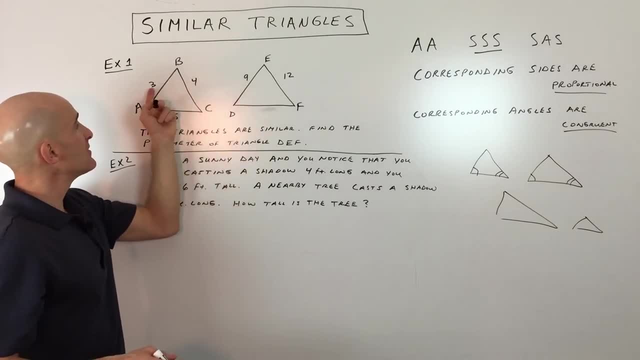 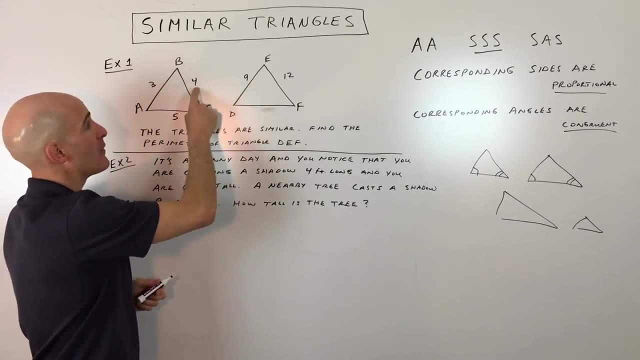 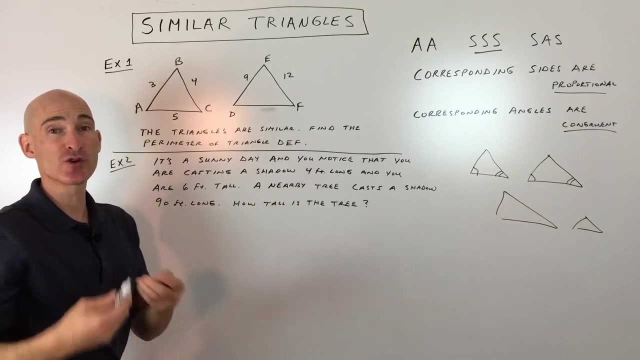 Okay. so now what we want to notice is that, see, if we were to match up these triangles, you can see three is to nine, okay, that's multiplied by three. right? four is to twelve. that's multiplied by three, five is to fifteen. so you can see that the scale factor is three. we're tripling, so we know that this side is. 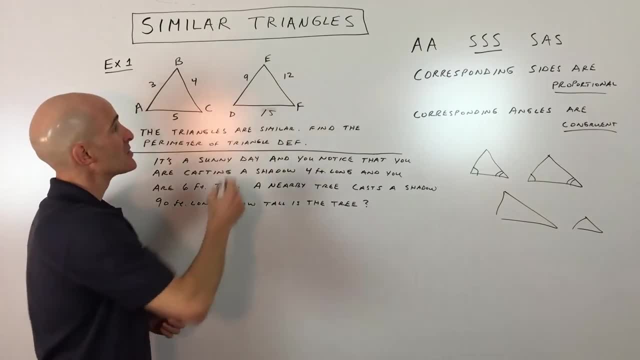 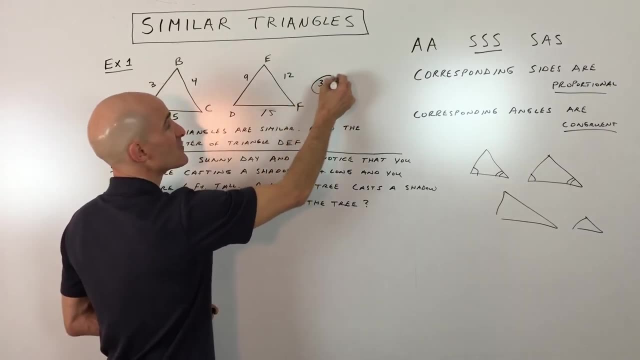 fifteen. we can then add up all three sides, so this is going to be- let's see, that's twenty seven plus nine, which is how much? thirty six. so the perimeter is just going to be thirty six units. the other way that you can do this problem is you could say: well, let me find out what the perimeter of this shape, this is. 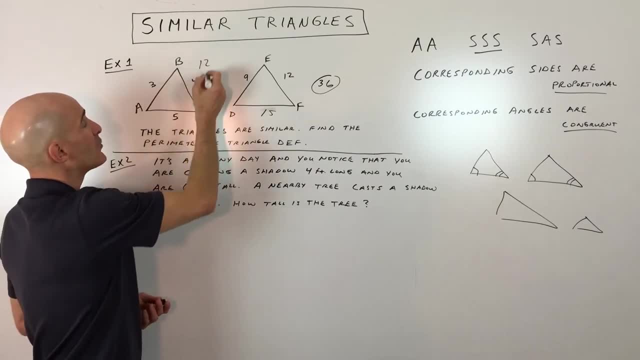 three plus four plus five, that's twelve. and if I know, the scale factor is three. I know I'm, you know, multiplying everything by three, the perimeter will also be three times larger. so we just have to take twelve times three, and that's thirty six. Okay, now let's go to a more challenging example. example number: 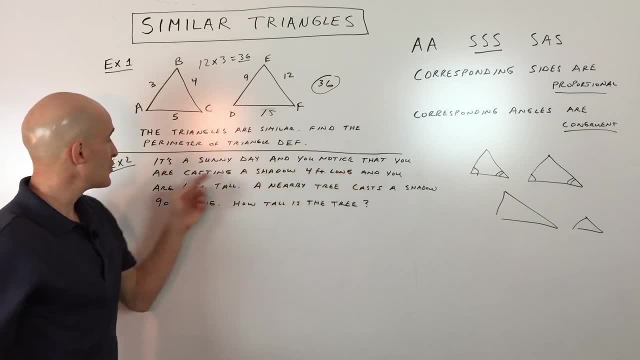 two. so it says it's a sunny day and you notice that you are casting a shadow that's four feet long and you are six feet tall. A nearby tree casts a shadow that's 90 feet long. How tall is the tree? So again, 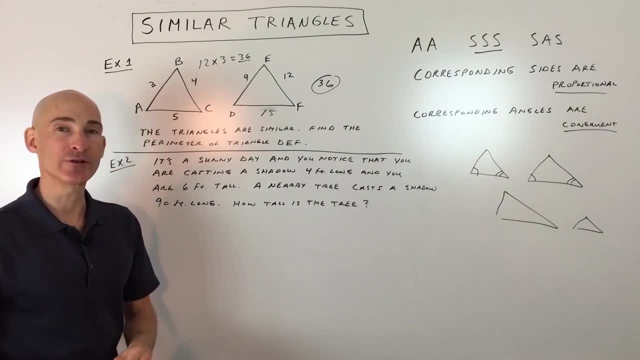 go ahead and pause the video, see if you can solve this problem, and then we'll go through it together. Okay, so the first thing that I would do on a problem like this is just draw a picture. so here's the Sun over here. okay, and let's just 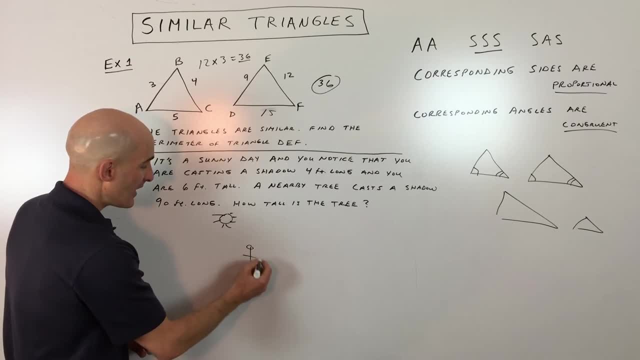 say that you're over here, okay, and you're casting your shadow like this, so you can see this is forming a triangle, actually a right triangle, okay. and here's the angle of the Sun like this, All right. And so here's the shadow. it looks like it's four feet long and you're six feet. 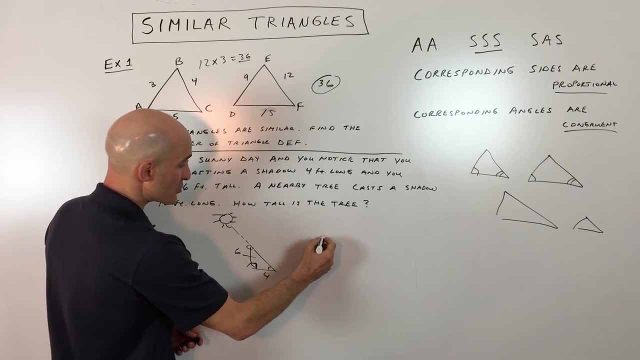 tall. Now over here we've got a tree that's a little bit larger- okay, see if I can draw a tree here for you- and it's casting a shadow that says it's 90 feet long. so this is 90, and we're trying to find the height of the tree. So what? 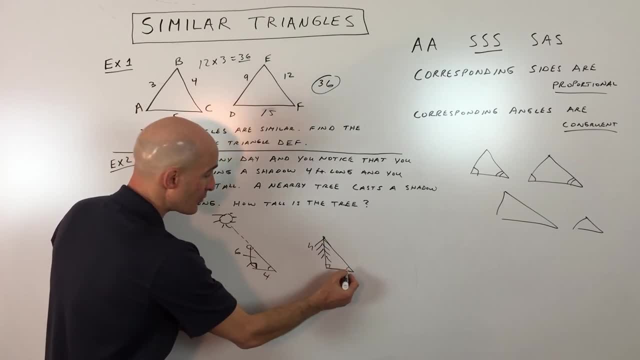 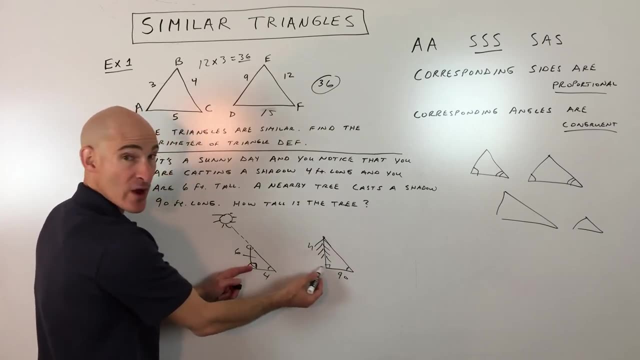 you'll notice here is that the angle of Sun is going to be the same in both of these examples. so we know that this angle and this angle are congruent. we're assuming that the tree is perpendicular to the ground and that you're perpendicular to the ground. so these are right angles. so you can see, we just 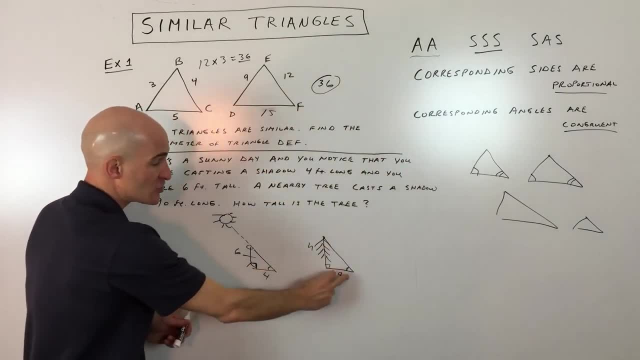 like we talked about over here, the angle angle. if we know two angles are congruent to two angles, then we know that the triangles are similar, which means that the corresponding sides are proportional. so all we have to do now is compare the corresponding sides so we know that your height is to the height. 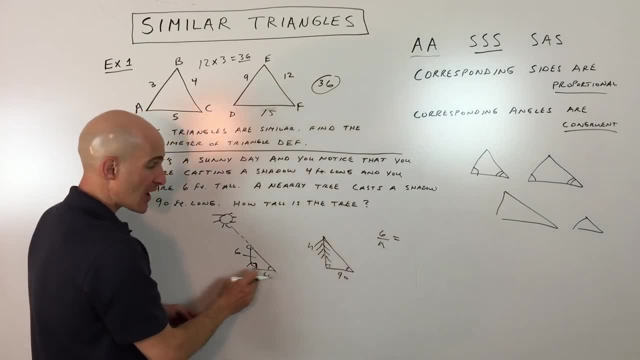 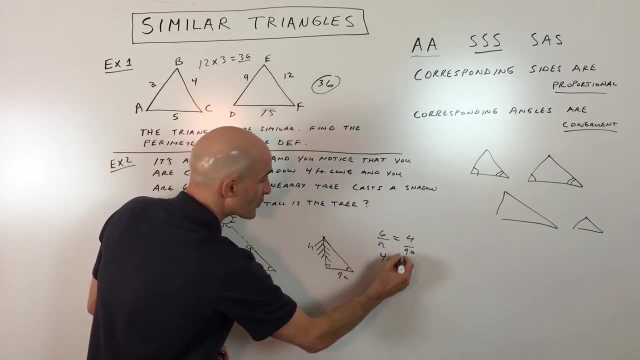 of the tree, so six is to H, as your shadow is to the tree shadow, so as four is to ninety, all we have to do now is cross multiply. so four times H equals a six times ninety, which is five hundred and forty, and then divide both sides by.